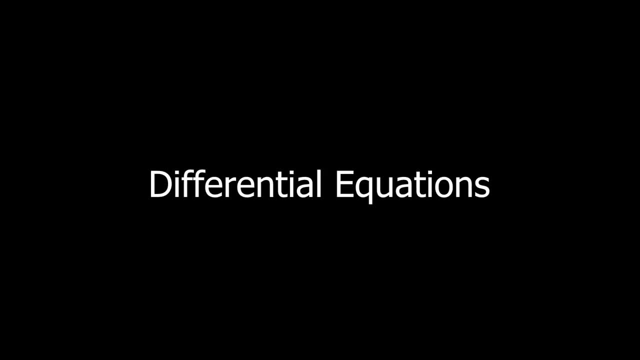 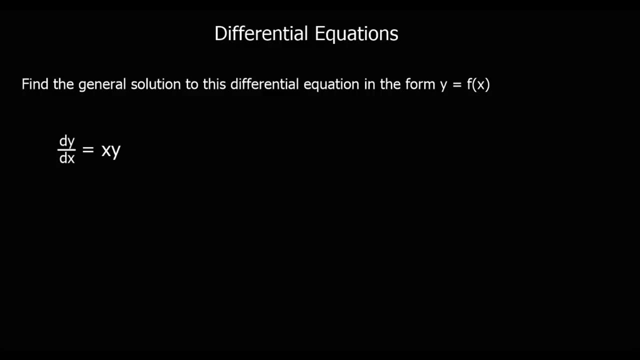 In this video we're going to look at differential equations. A differential equation is an equation, so it's got an equal sign with a derivative in it, with a dy dx or a dy dt or a dx dt or dx dy, so some kind of derivative within the equation. So here we've got dy dx equals xy. 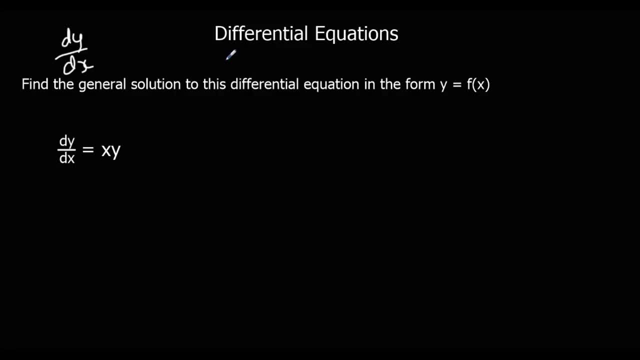 so we've got a dy dx in an equation, so it's a differential equation. We're being asked to get it in the form y equals f of x. so we want to get rid of the dy dx. To do that, what we do is we split. 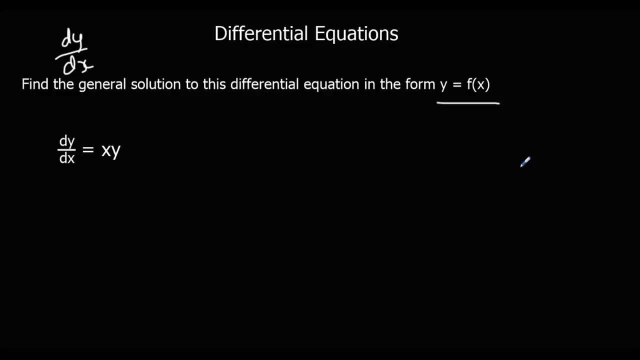 up the x's and the y's so we separate out x's on one side and y's on the other side. So here we've got dy dx. so if we imagine that we times both sides by dx, we can take the dx to the other side and have dy. 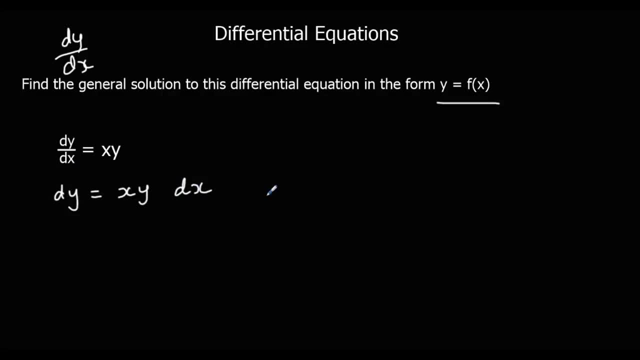 on one side and dx on the other side, Then we need to get all the y's with the dy and all the x's with the dx. So if we divide both sides by y, we'll get one over y. dy equals x- dx, So we've split all. 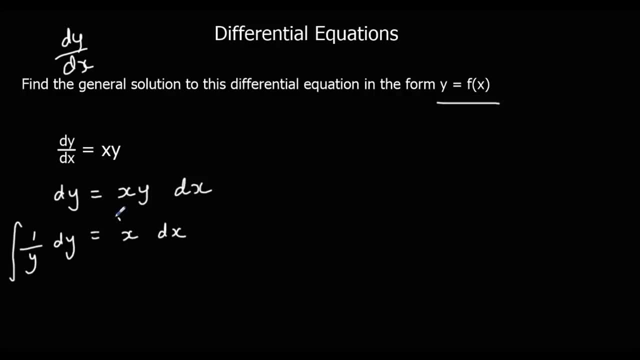 the y's onto the left side, all the x's on to the right side, and now we can integrate both sides. so integrating one over y with respect to y is ln y and the integral of x with respect to x is x squared over two or half x squared. We need to plus c, but we only need to plus it to one side. 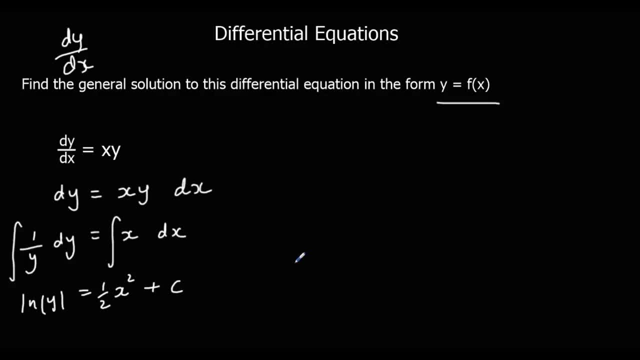 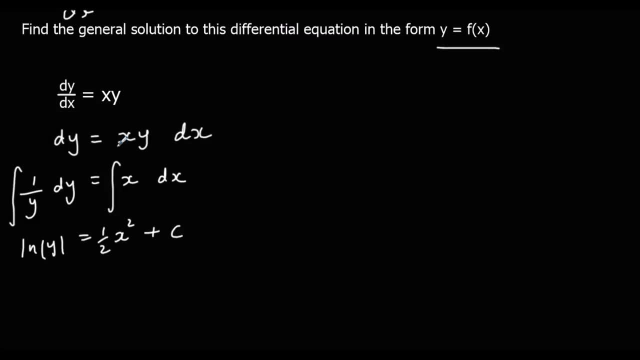 because if there's a constant on both sides, we can take one of them over to the other side. so there's only one c and we need to get it in the form y equals f of x. so to get rid of lny, to get rid of an ln, to get y by itself, we e both sides. so y equals e, half x squared plus c. 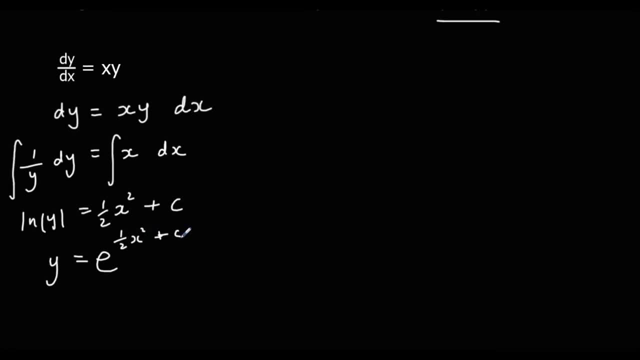 that is an answer. we can simplify that a little by changing it to e, half x squared times e c. so when you multiply powers, when you multiply two indices, you add the powers and we can change e c to a different constant. so we'll call that a, so we'll have a. 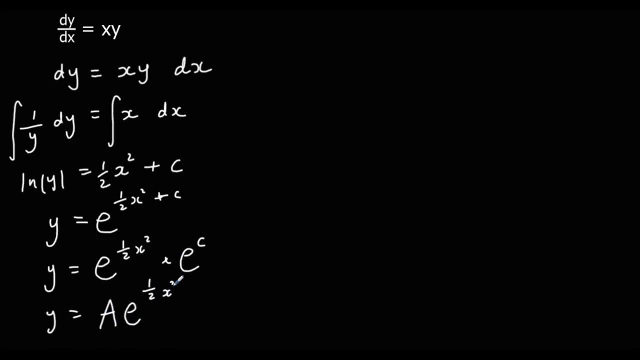 c and we'll call that a. so we'll have a c and we'll call that a c and we'll call that a c. and times e, half x squared. okay, here's another question. so again, find the general solution for this differential equation in the form: y equals f of x. so again, we're gonna split up. 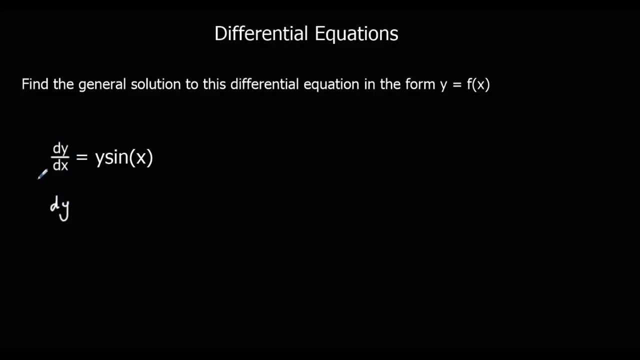 the x and the y and we're gonna get all the wires on the left side and all the X's on the right side. So again, we divide by y and have 1 over y. dy equals sine, x, dx And we're going to integrate both sides, which will give us ln. y equals integrating sine gives us negative. 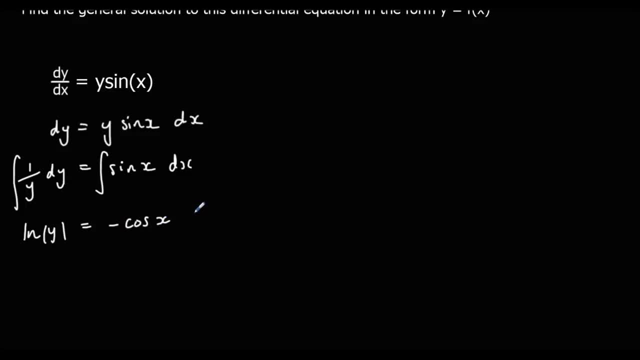 cos, so negative cos x and plus c. So again we're going to e both sides to get rid of the ln. So that'll just give us y equals e to the power of minus cos x, plus c, And again we will change it to e to the power of c times e to the power of minus cos x. 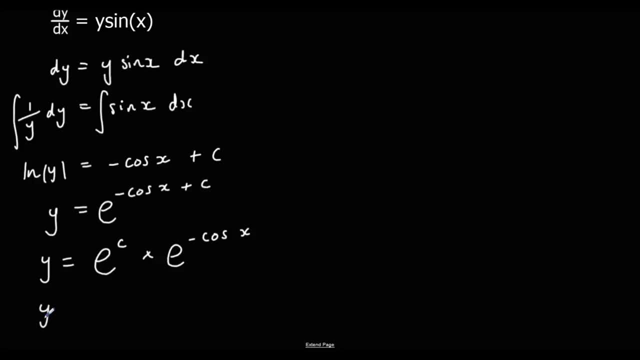 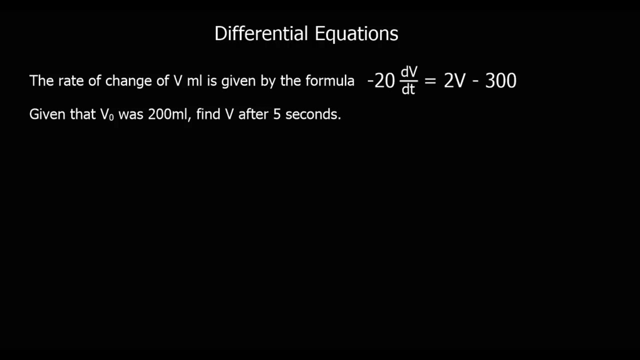 x. e to the power of c is just a number and we're going to call it a, So a e minus cos x is our answer. OK, here we're going to look at a differential equation in context. So we're told the rate of change of v volume, milliliters, is given by the formula minus. 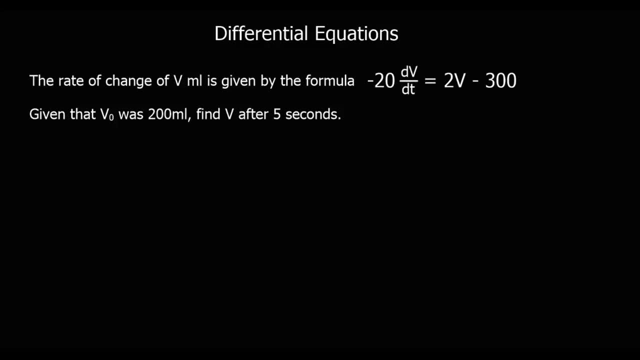 20 dv, dt equals 2v And we're told that at v0, so v0, the volume at time equals 0. So when t equals 0, v is 200.. So we're going to be able to use that information to find c this time. So what we're? 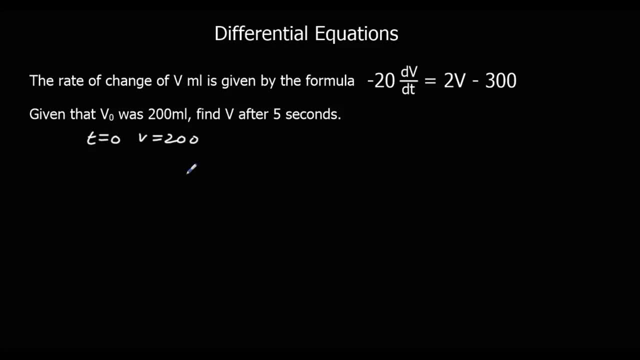 going to do? we're going to split it up, So get all the v's on one side and the t's on the other, So I have minus 20 dv, And then I'm just going to divide it by 200 over 200 minus 300.. So that gives me negative. 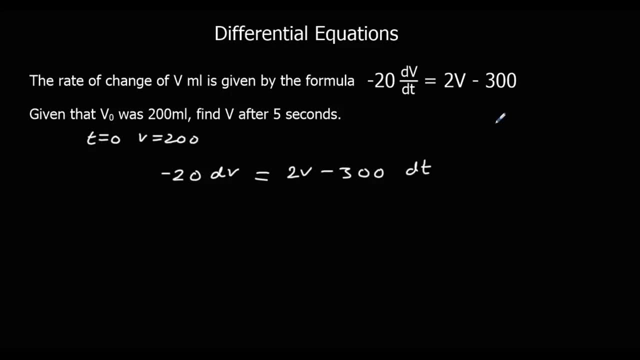 0, minus 300 dv. dv, dv minus 300 dv. So all the v's, all the v's to the right and the dv's, all the v's, all the v's to the left side. There are no t's, so we're going. 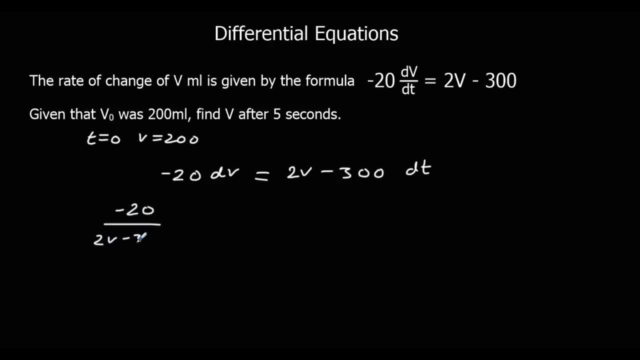 to divide by 2v minus 300. Over 2v minus 300.. And we're just going to have one on the t side, So we're going to integrate minus 20 over 2V minus 300. with respect to V. 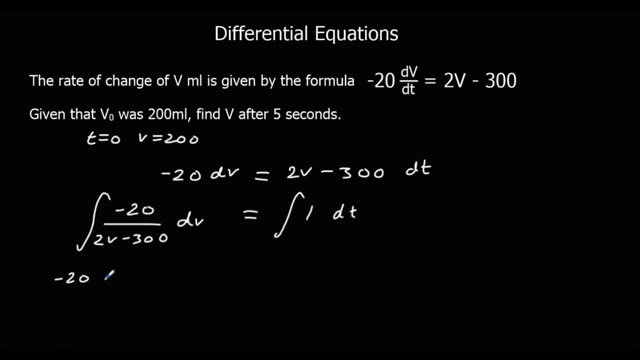 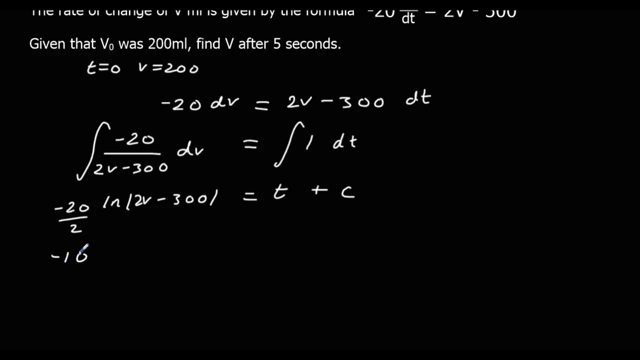 So we will have minus 20 ln 2V minus 300 and divide by the bracket differentiated, which is 2.. And that's going to equal 1. integrated with respect to T is T and we'll plus C. So, simplifying, we've got minus 10 ln. 2V minus 300, equals T plus C. 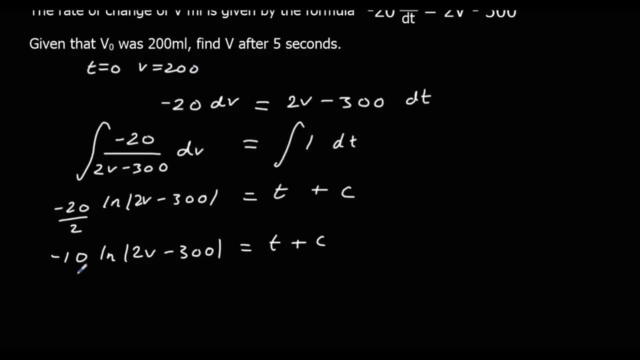 When T is 0, V is 200.. So we'll substitute those in and we'll find C, So V is 200.. So 2V minus 300 is 100.. And then 100 minus 200.. 10 ln. 100 equals C. 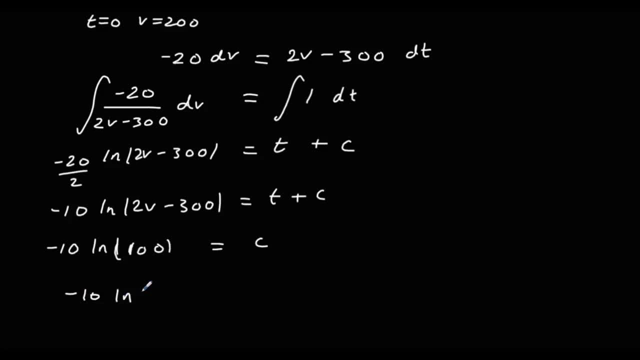 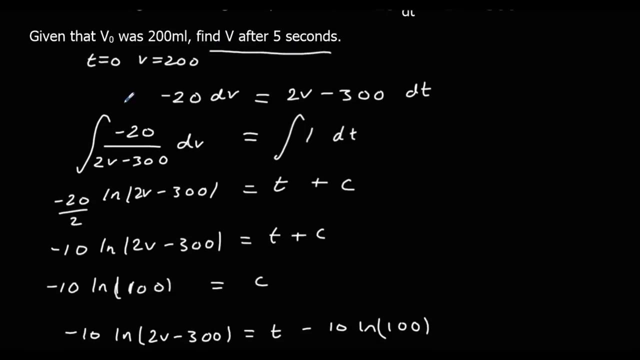 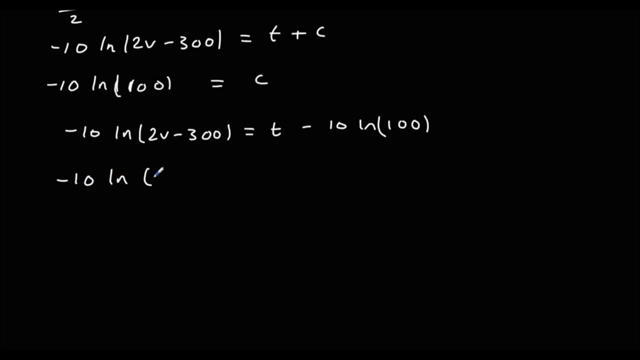 So we've got minus 10 ln 2V minus 300 equals T minus 10 ln 100.. And we want to find V after 5 seconds. So when T is 5, what is V? So minus 10 ln 2V, minus 300.. 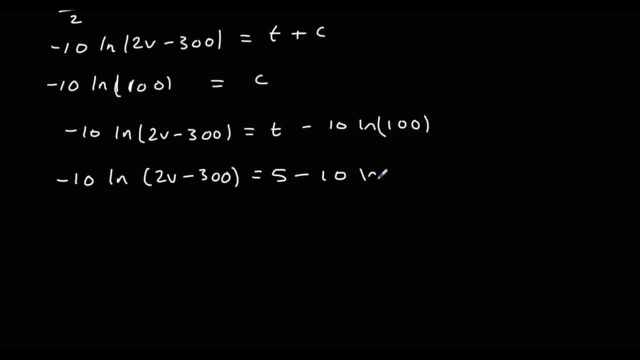 100 equals 5 minus 10 ln 100. So we need to get V by itself. So we'll divide by a negative 10.. Divide every term by negative 10. Which gives us negative half plus ln 100. Then we're going to E both sides to get rid of ln. 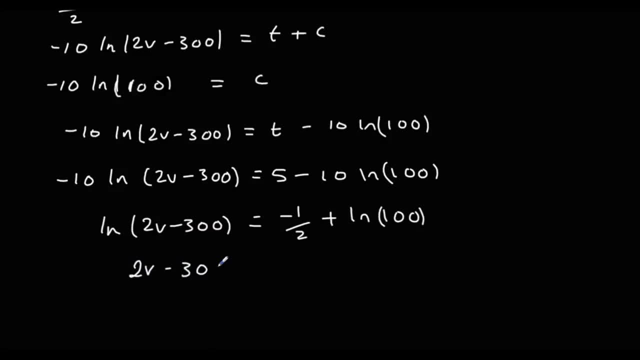 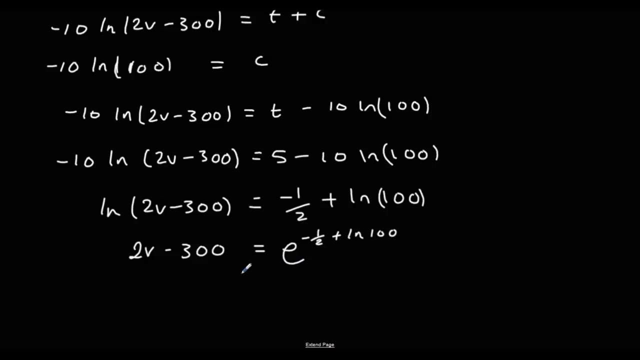 We're going to E. So 2V E minus 300 equals E to the power of minus a half plus ln 100.. We could simplify this, But let's just get V by itself first. So plus 300 and divide by 2.. 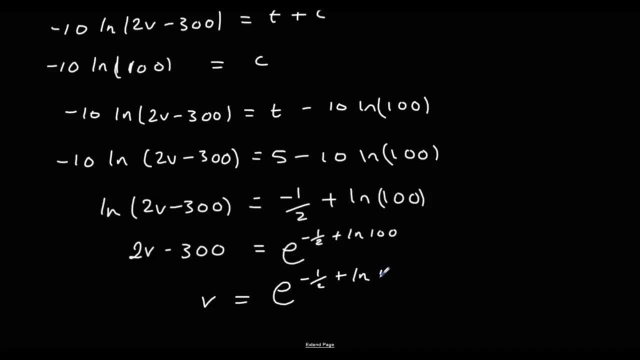 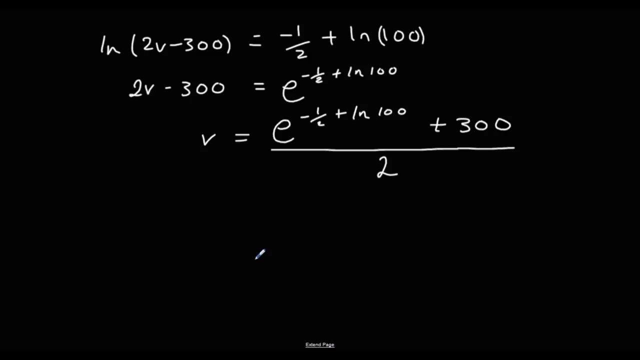 So E to the power of minus a half plus ln, 100 plus 300.. 0 all over 2. so we're going to give our answer as a number so we don't have to worry about simplifying the e term. so let's put it in the calculator and we should get 180. 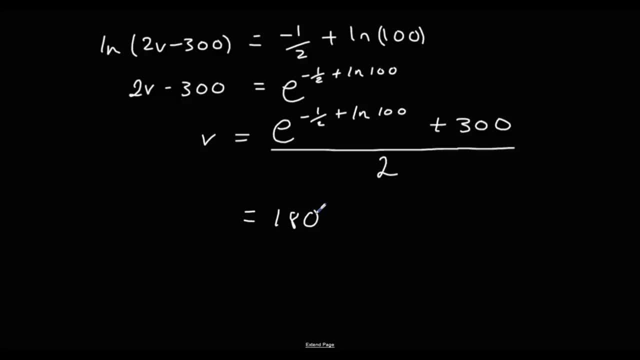 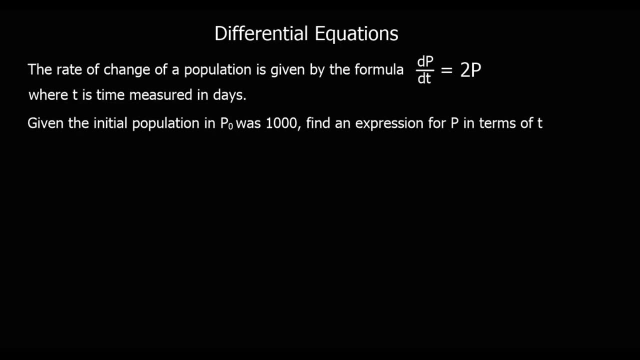 milliliters to three significant figures. okay, here's another question. pause the video, give it a go and press play when you're ready to go through the answer. okay, so we've got the rate of change of a population this time and we've got dp dt. 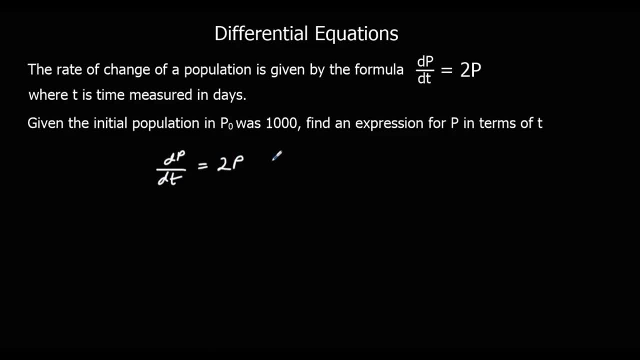 equals 2p. so we're going to split up the p's and t's so we'll have dp or 1 over 2p. dp equals 1, dt. we're going to integrate both sides, so 1 over 2p is going to become ln. 2p divided by the bracket differentiated.